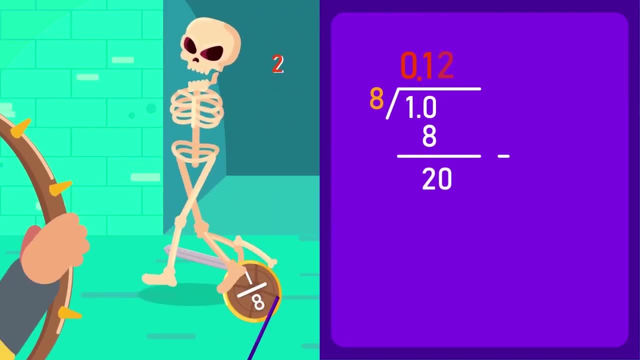 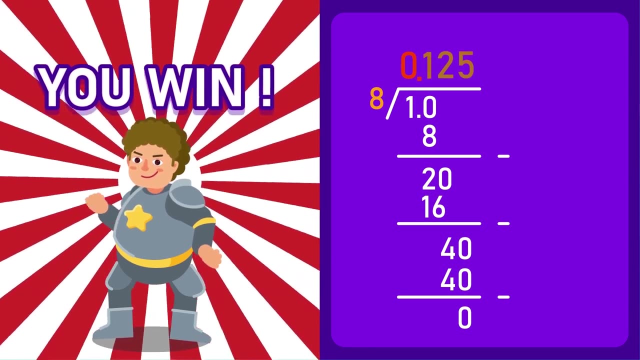 example, When we divide 1 by 8, we get 0 as a remainder and 0.125 is the terminating decimal number that has a finite number of digits. that is three numbers after the decimal point. Now let's take another number: 1 over 3.. If we see this example, the division never ends. The remainder, again and again, appears to be 1, and the quotient keeps on repeating as 0.33333 and so on. Therefore, a decimal number where the number of digits after the decimal point is infinite is called a non-terminating decimal. 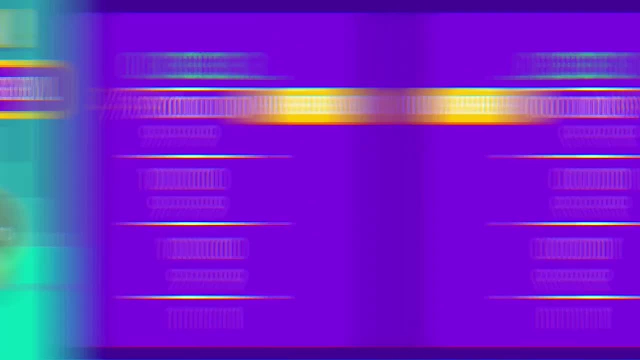 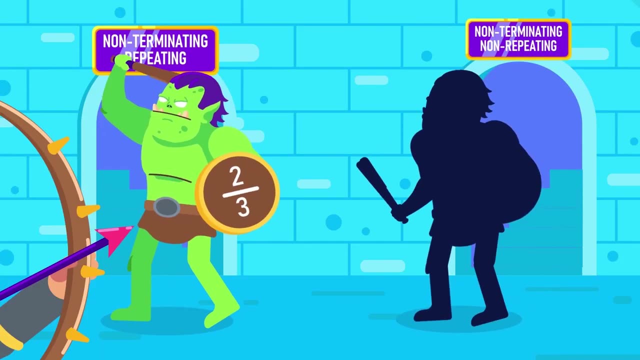 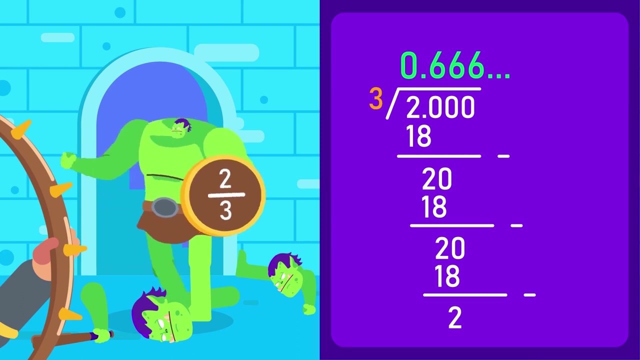 number, a decimal number that never ends. The non-terminating decimal number also has two types: repeating And non-repeating decimal numbers. When we convert 2 over 3 to a decimal number, it will be a non-terminating repeating decimal number. that is, 0.666666 and so on That will 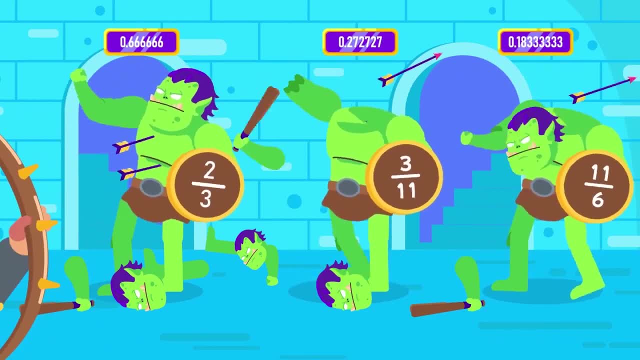 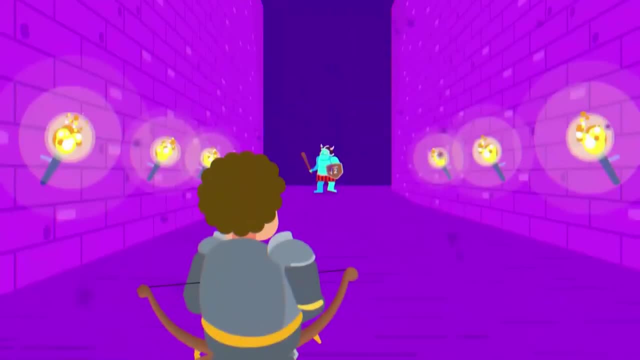 be similar to 3 over 11 and 11 over 6, which give the result of repeating decimals that never ends. They are all non-terminating repeating decimal numbers, but the case is different with the square root of 2,, which is an irrational number. It will give us the answer to the question. 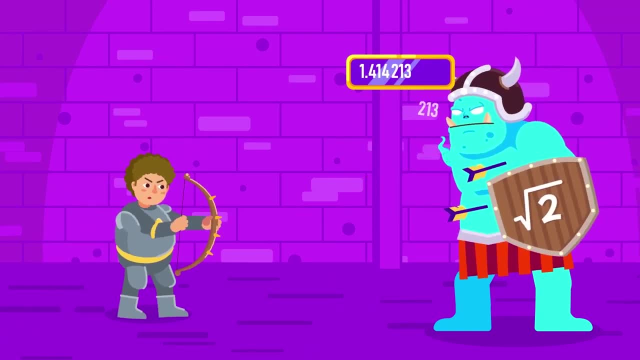 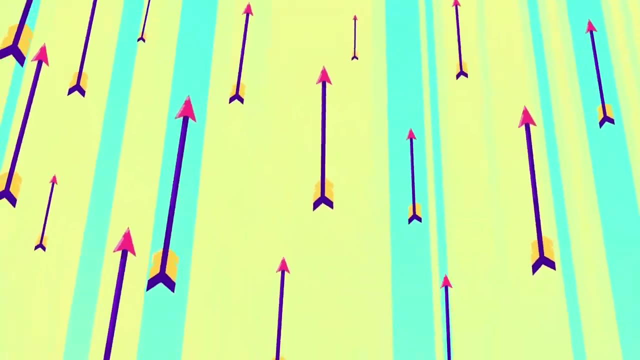 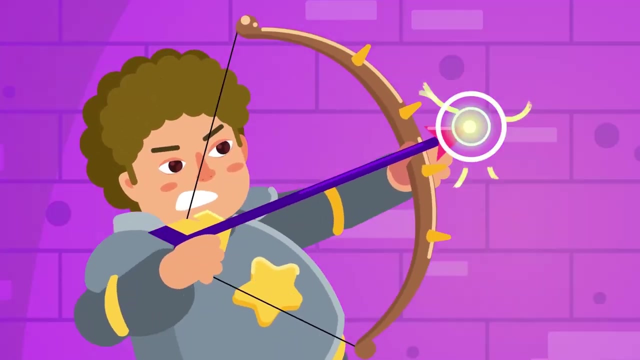 1.4142135623 and so on. We will soon notice that, for this case, the digits after the decimal point are non-terminating and non-repeating. Hence this is the second type related to non-terminating decimals. The square root of 3 is also an irrational number. 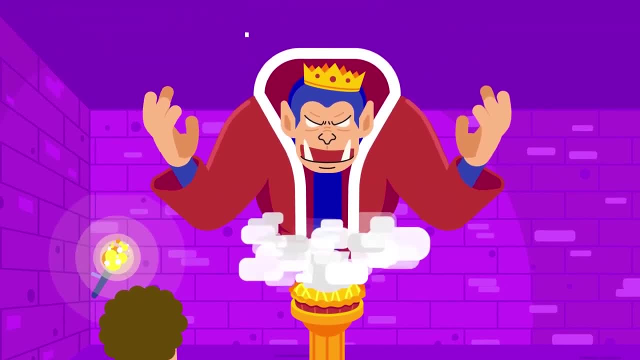 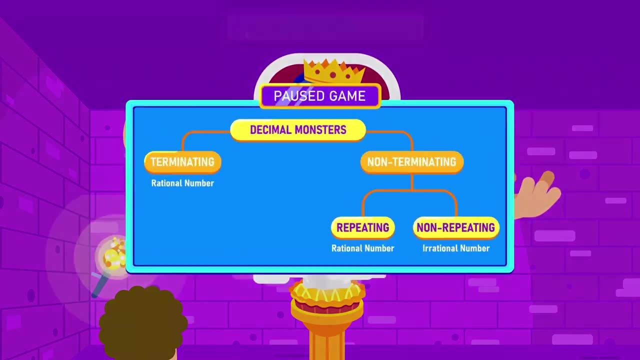 How about pi? Yes, definitely not the kind of pi that you expected. It is an irrational pi that gives you non-repeating decimals. It is an irrational pi that gives you non-repeating decimals. Here is a diagram showing the types of decimal numbers that we just studied. 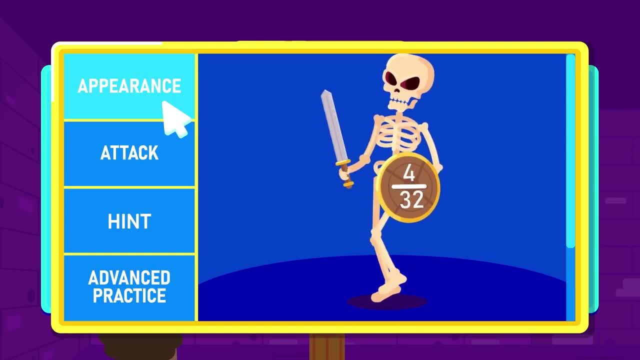 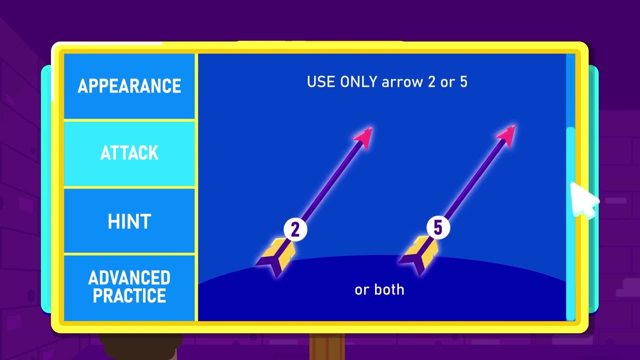 Now how can you tell if a fraction is a terminating decimal? We can resolve the denominator of the fraction into its prime factors. If the prime factors consists of only 2 or 5 or both, then the fraction will absolutely be a terminating decimal. This will be super. 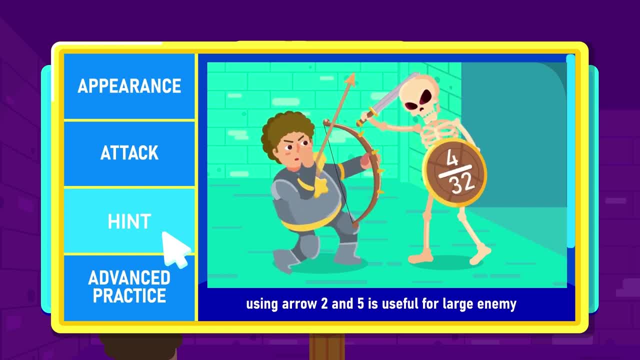 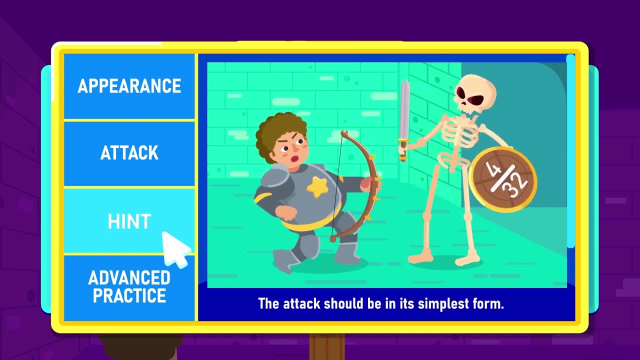 helpful when you're encountering a large fraction and not sure if the remainder of the long division ever yields the same number. If the denominator of the long division yields the same number, then the fraction should be in its simplest form Before we start the factorization. once simplified, you can factorize the denominator.